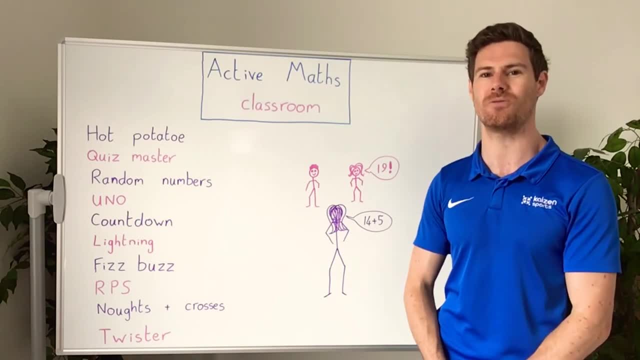 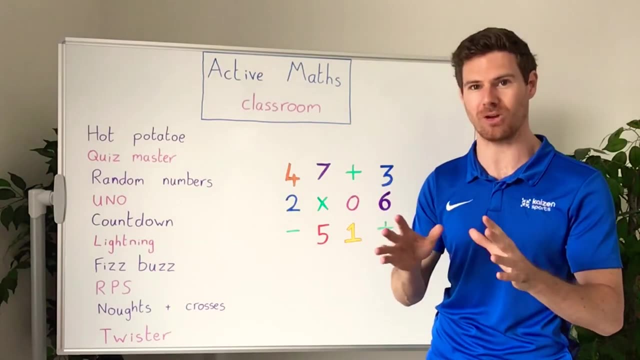 and watch their excitement for mental arithmetic go through the roof. In the game Random Numbers, you're going to laminate some numbers and some functions. Make sure you've got lots of them and put them all out across your desk. Now the children are going to work in pairs. they're going to come up to the desk. 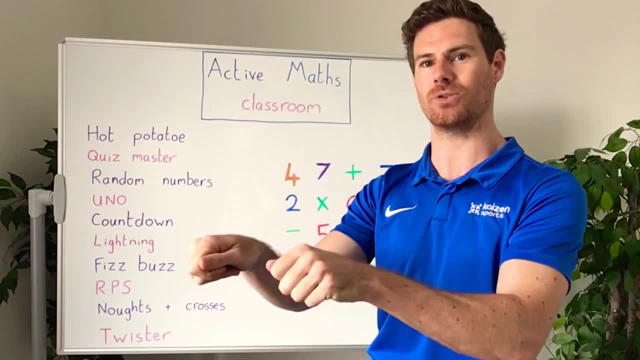 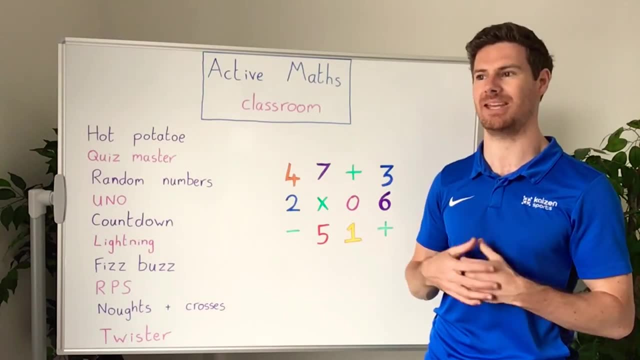 and they're going to select three numbers and two functions to take back to their desk. Once everybody's done that, you're going to call out an answer, So your answer might be 17.. The children then have 30 seconds to work together to try and use the numbers and the 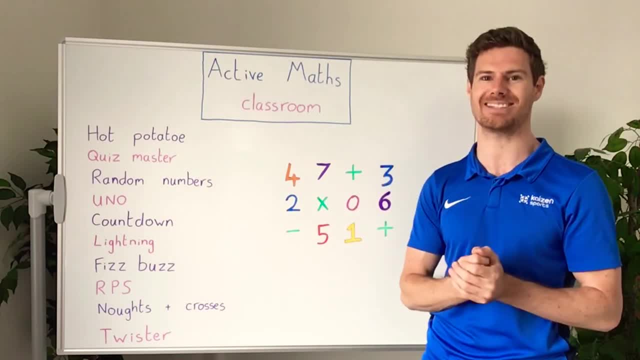 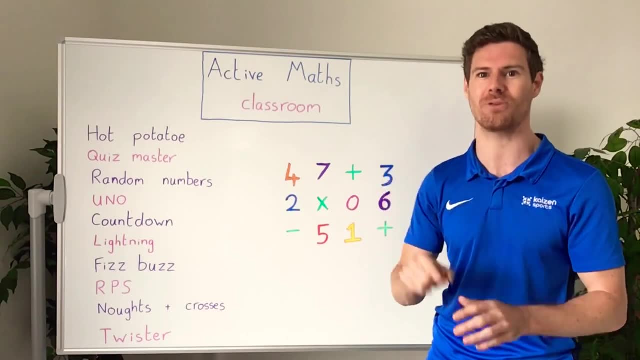 functions to get either the answer or as close to the answer as they can. This is great for teamwork, and children get a real rush if they're the first ones to be able to work together and solve the problem. In the game Over Uno, you're going to get into your table groups and select. 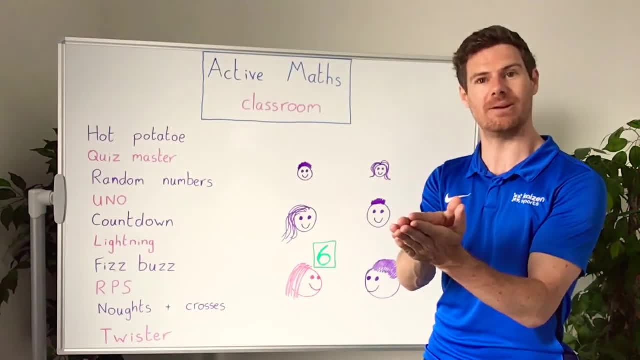 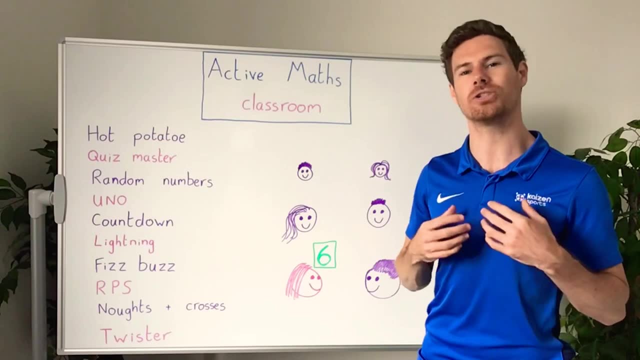 one leader who's going to start with a deck of cards, Now one at a time. they're going to turn the card over and then present it to the group, So they'll be presented with a colour and a number. Now the colour denotes the action that they have to take, So a red colour might be jump. 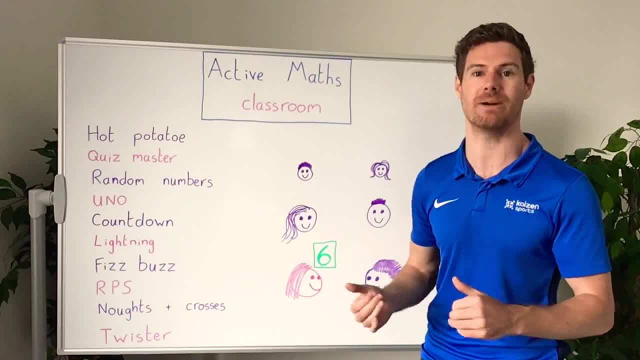 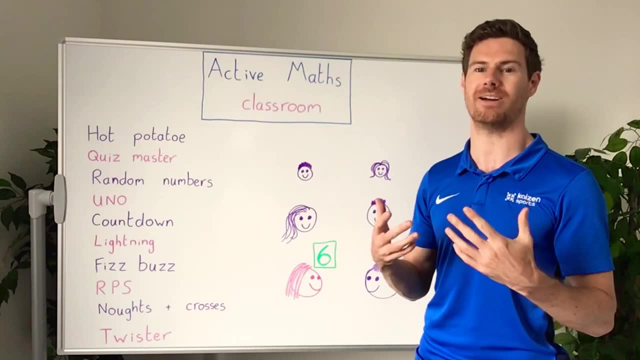 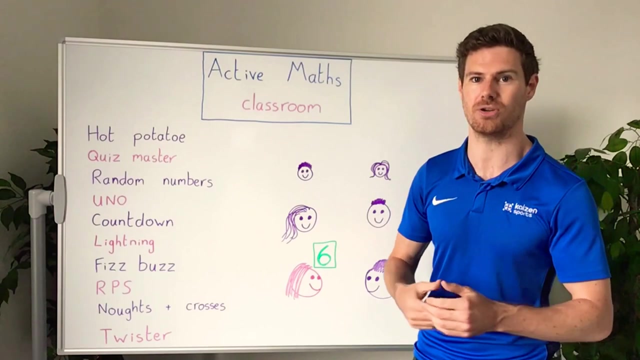 yellow might be squat, blue might be spin around and green might be to hold the balance. Make sure that with the numbers, you're linking them into your outcome. For example, if you're working on the five times table and six is shown, six would be the number that you then times by five. So the first person to 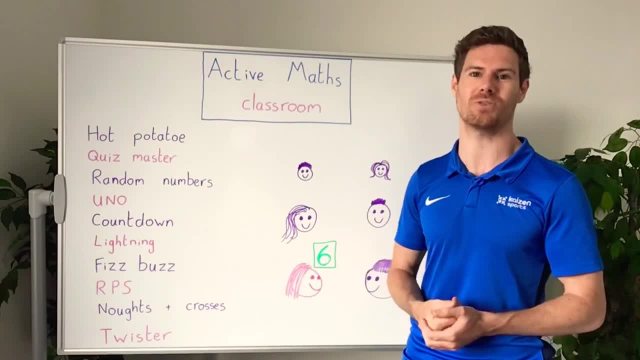 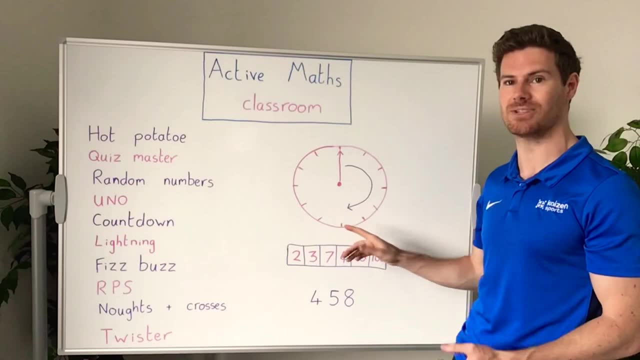 green, hold the balance and shout out 30 would then score the point. In the game of Countdown, children are going to start with a whiteboard and they have 30 seconds to use the numbers and try and reach the target answer, just like in the TV show. Now they must. 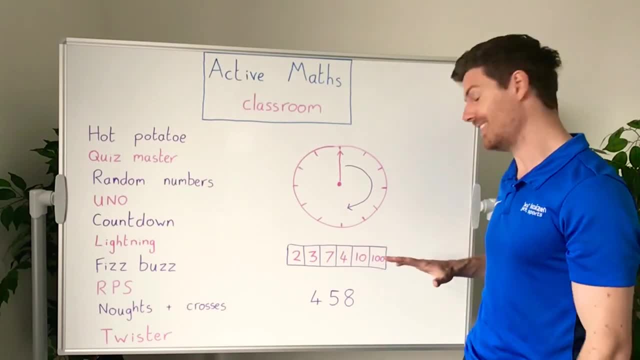 show they're working out, because we know what they're like In the beginning. you're going to pick the numbers and the target answer and then you're going to show them what you think they're working out, because we know what they're like In the beginning. you're going to pick the numbers and 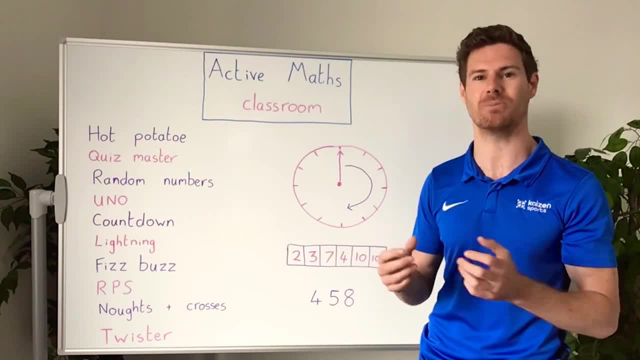 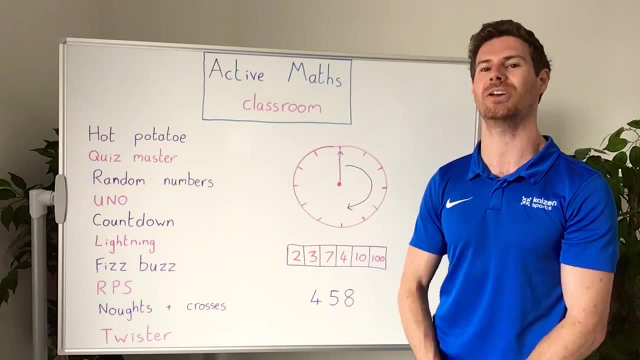 the target answer and eventually, as time goes on, we can let children pick the numbers once they get used to the structure. Make sure you play the theme tune in the background to crank up the excitement and, as always, link it to your learning outcome. The game of Lightning is immensely. 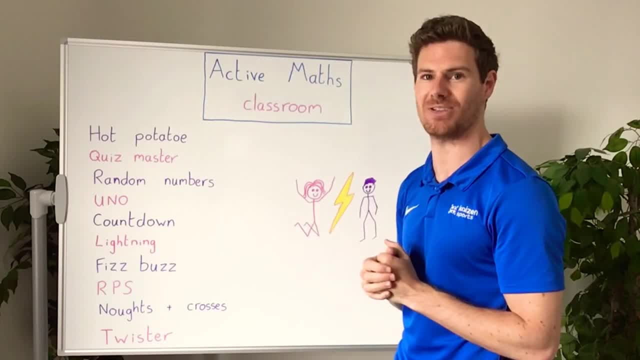 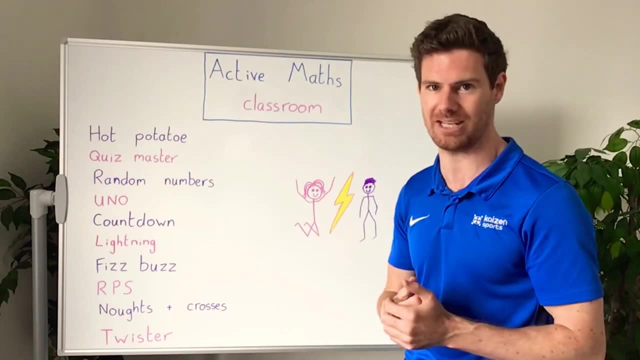 popular Now. children are going to pair up and then face off against each other. In this game, the action that they need to fulfill is a jump when they hear a multiple of three if you're working on the three times table. So they're going to face up against each other. 17,. 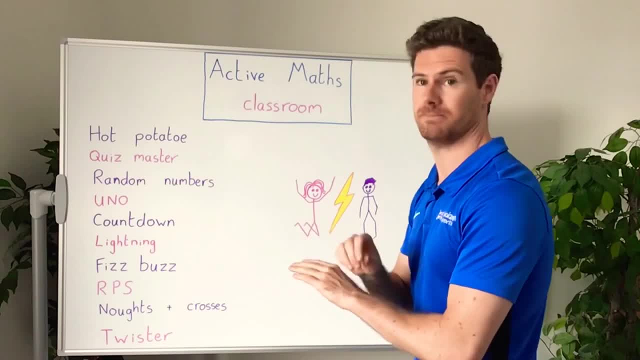 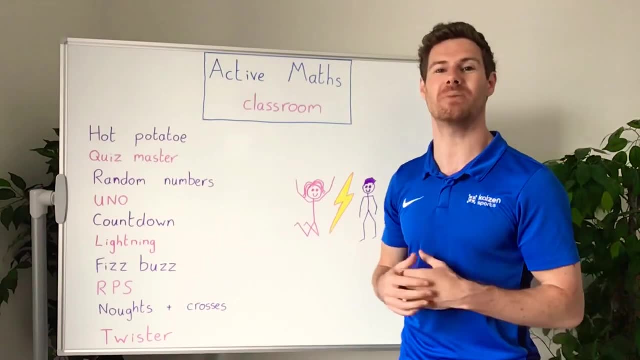 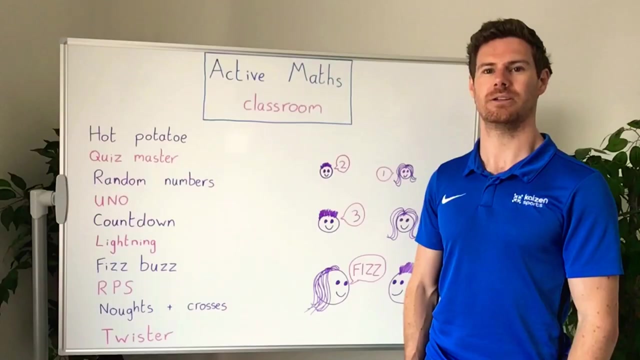 nothing happens 22,. nothing happens 9.. The first person to jump up scores the point, because 9 is a multiple of three. Make sure you mix up the actions as well. this could be anything from a jump, a twist and a squat right through to a mini dance-off. Table groups are perfect for fizzbuzz. 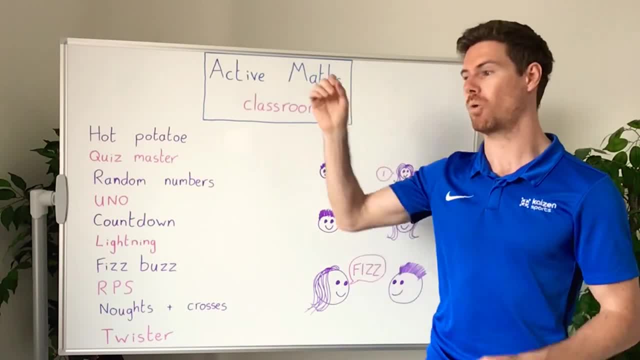 so children are going to go around and count the next number in the sequence: 1,, 2,, 3,, 4, 5, 6,, 7,, 8 and so on. Now, if you're working on the four times table, 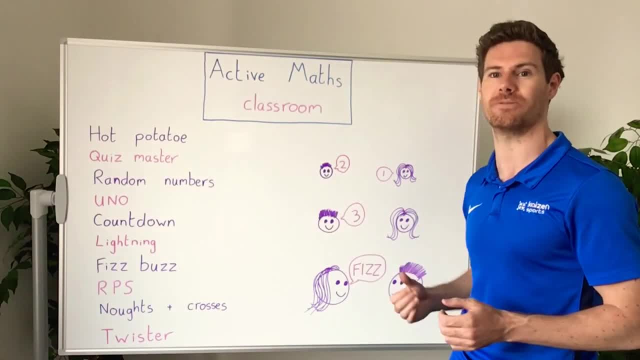 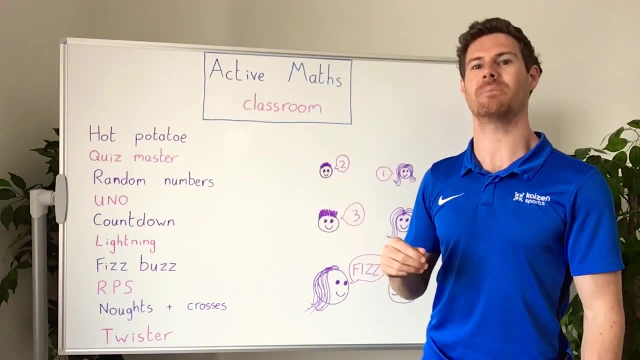 instead of saying four or the multiple of four, you're going to say the word fizz. So, as you can see in this example, 1, 2,, 3, fizz, 5, 6,, 7, fizz, and so on. Now you can make the game even more. 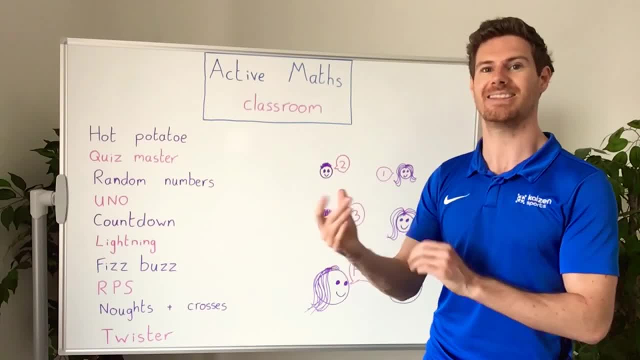 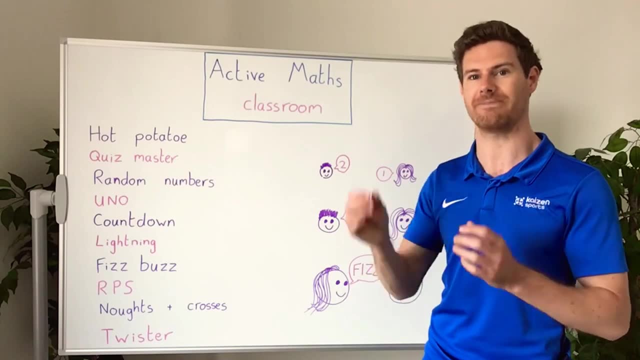 difficult by saying the word fizzbuzz instead of just fizz. This means that you carry on playing the game, but the momentum shifts back the other way. This is great for learning. times table very quickly and forces children to think and plan ahead. Rock paper, scissors, maths is probably. 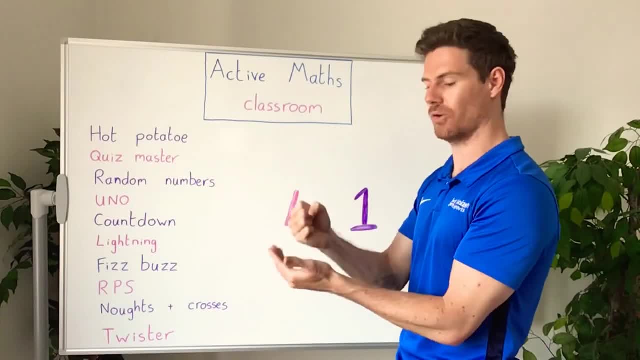 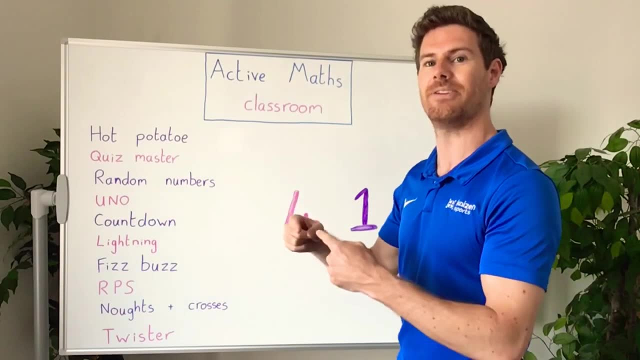 the easiest way to get the most out of a game You're going to get with a partner and instead of going rock paper scissors shoot and showing rock paper scissors, you're going to show a digit: 1,, 2,, 3,, 4 or 5.. The first person to add up the total number of 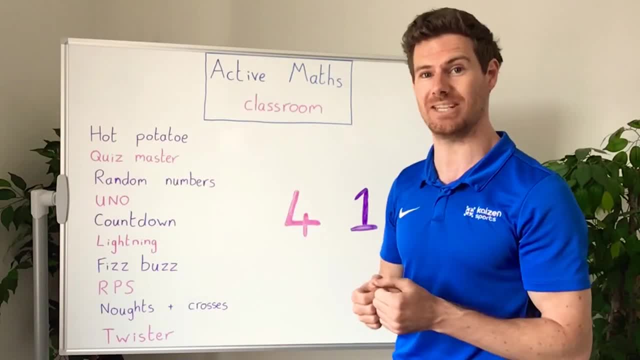 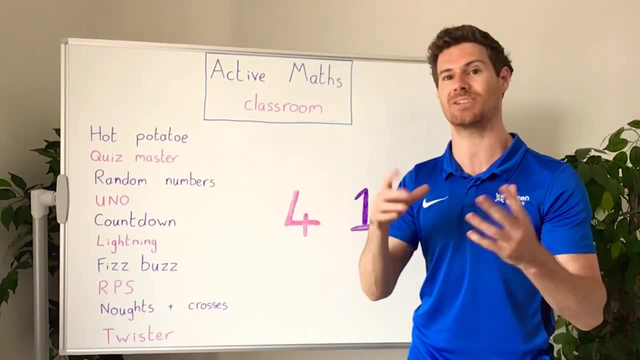 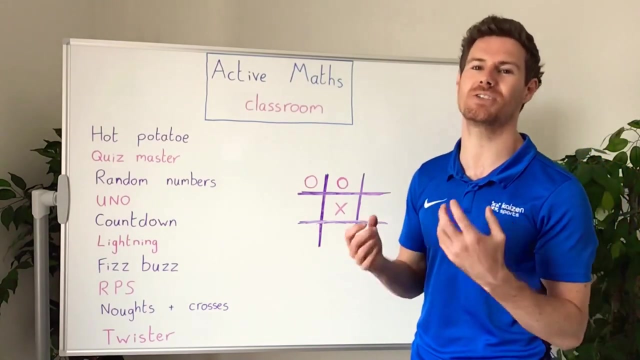 fingers on show is the winner. Now you can make this game twice as difficult by playing the game with two hands and adding up the total, or you can also throw in some times tables in there, if that links with your outcome. It's a dead easy game and children love it. A partner and two dice is 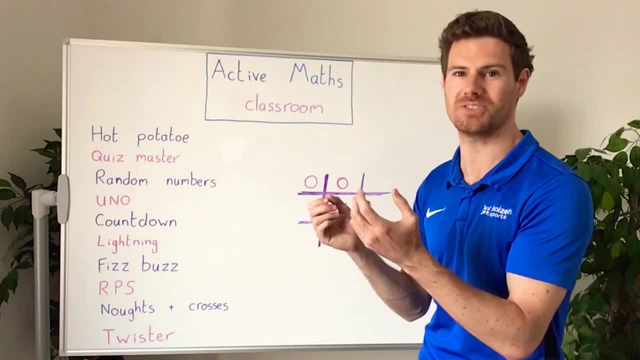 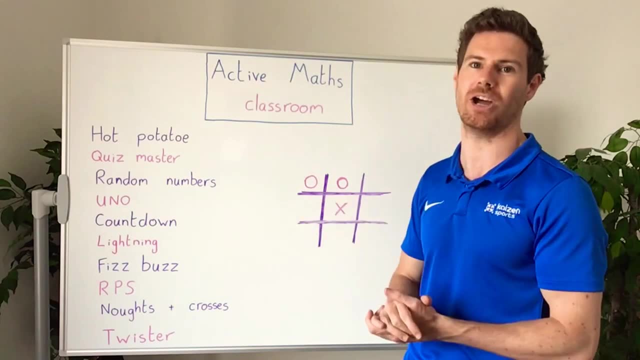 all you need for noughts and crosses. You're going to roll the dice and you have 10 seconds to correctly add up the two numbers. If you can't do it within 10 seconds or you give a wrong answer, you then forfeit your go and you can't put a nought or a cross down. It's your partner's. 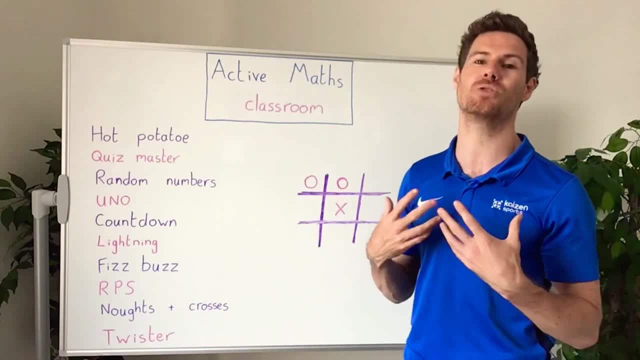 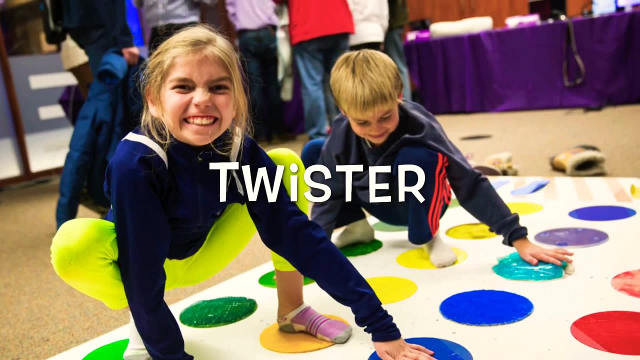 turn to go. Three in a row wins. and, as always, make sure you tweak the focus to work on multiplication, subtraction, number ponds, whatever your focus may be. And finally, we have Twister. Now you can either use the official board game or you can pop to.